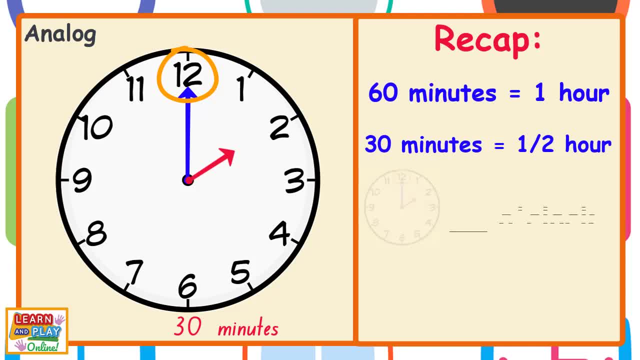 Remember when the minute hand is pointing at the number 12, we say it is something o'clock. Also, remember that when the minute hand is pointing at the number 6, we say it is half past something. So that means that half a rotation is equal to 30 minutes. 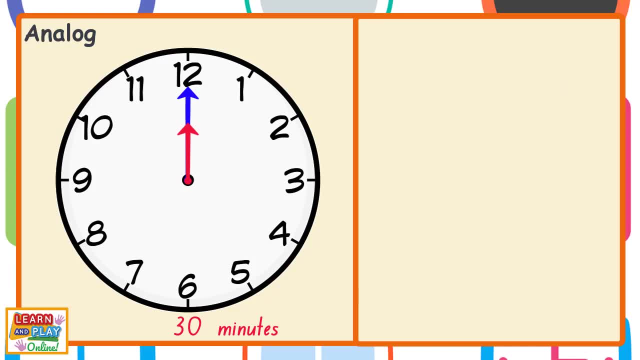 The time on the clock face now says 12 o'clock. Now watch what happens when the minute hand only travels a quarter of the way around the clock. As you can see, the minute hand is now pointing at the number 3.. When the minute hand is pointing to the number 3 on an analog clock. 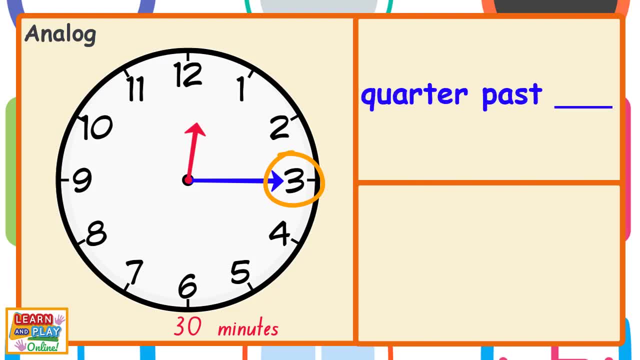 we say it is quarter past something as the minute hand only travelled one quarter of the way around the clock. If you look at the hour hand, it has just passed the number 12.. So this means the time on the clock is quarter past 12.. 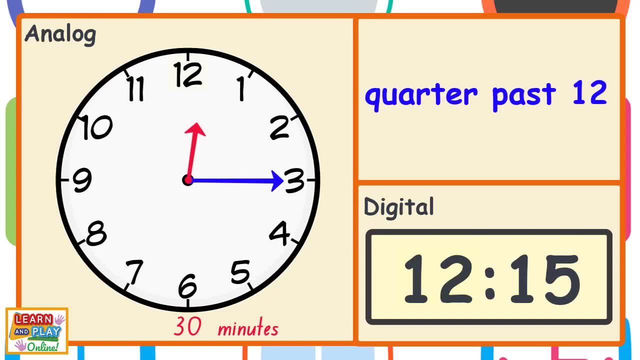 On a digital clock it would read 12.15.. Because we are in the 12th hour and a quarter past means only 15 minutes has passed the hour, since 15 minutes is a quarter of 60 minutes, Now that you have learned how to read quarter past times. 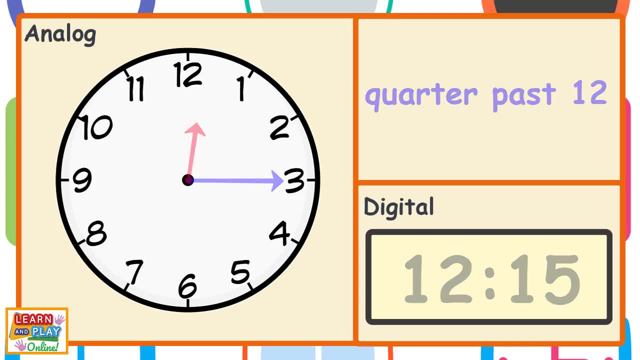 let's practice reading the times on the clock coming up So we can see that the minute hand is pointing at the number 3, so it is quarter past something. The hour hand is just past the 10,, so that means it is quarter past 10,. 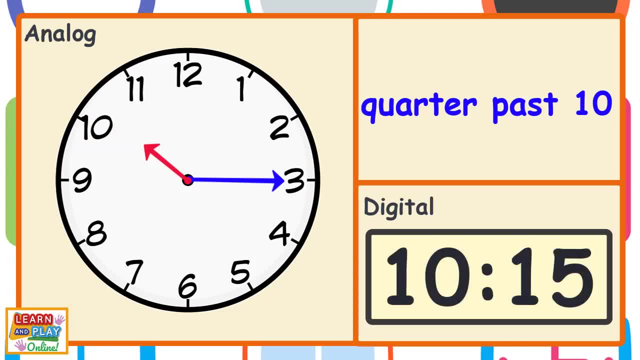 or 10.15.. The minute hand is pointing at the number 3, so it must be quarter past something. The hour hand is just past the number 7, so it is quarter past 7, or 7.15.. The hour hand is pointing at the number 7,. 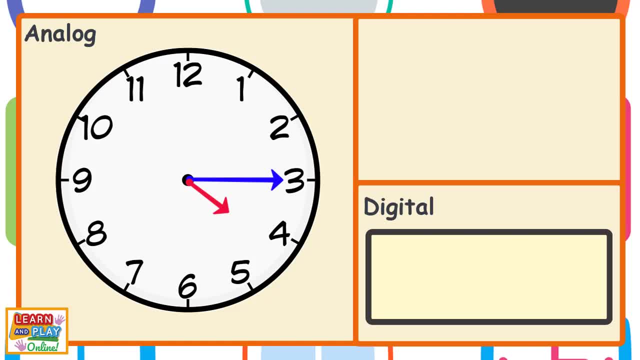 so it is quarter past 7, or 7.15.. The minute hand is pointing at the number 3, so it must be quarter past something, And the hour hand is just past the number 4, so that means the time is quarter past 4,. 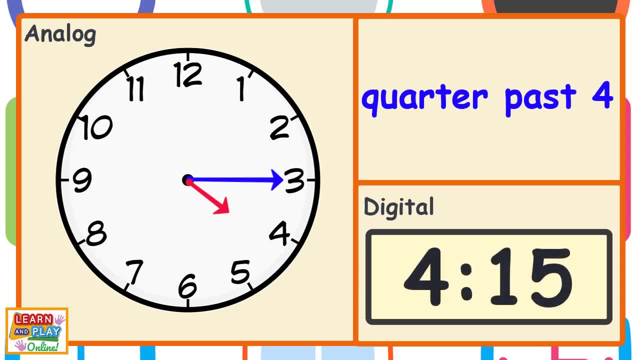 or 4.15.. The second quarter past something carpet or 9.15.. The third quarter past something slow, so maybe 10 minutes or so, And the third quarter not is Rota passed 9 or 9.15..